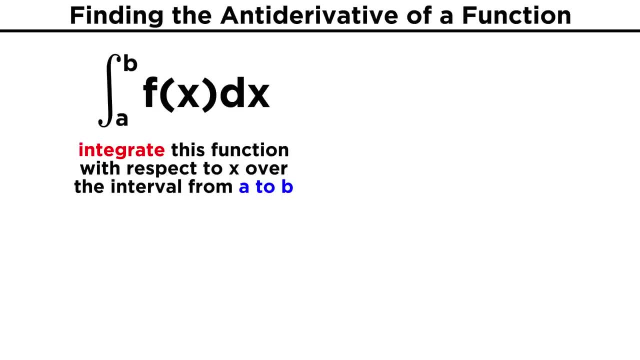 If we want to integrate this function, f of x over the interval from a to b, that will be equal to f of b minus f of a, where the upercase is a, Why lowercase f represents the antiderivative of the function. 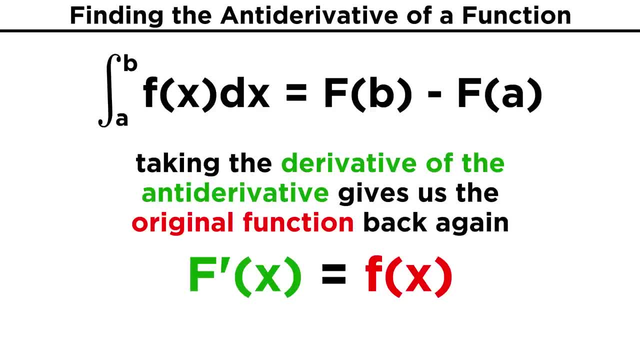 So what's an antiderivative? Well, that's a function for which if you take the derivative, you get the original function, kind of like how squaring a square root gives you what's inside the root. So capital F is the antiderivative of lowercase f, because big F prime equals little f. 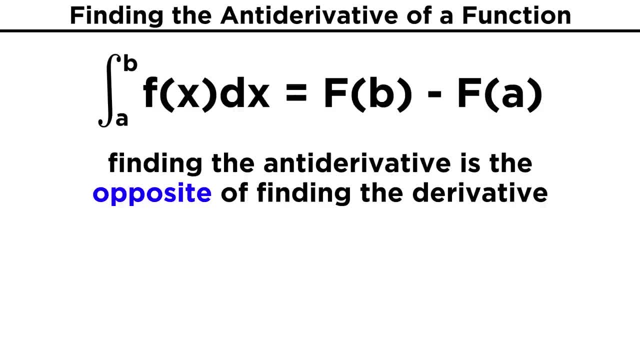 In order to get an antiderivative, we are going to have to employ precisely the opposite algorithm of the one that is employed during differentiation. Remember that when we take a derivative, we bring this exponent down here and then reduce the exponent by one. 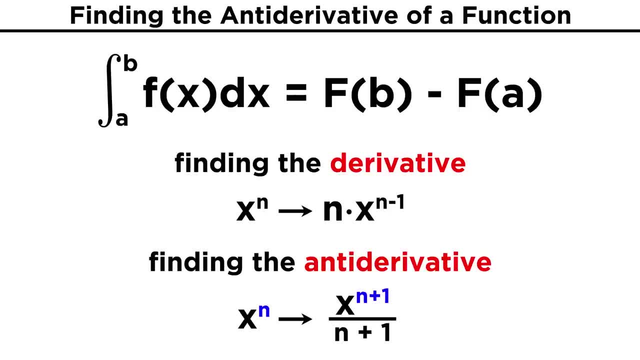 That means that to get an antiderivative we have to increase the exponent by one and then divide the resulting term by the new exponent. For example, to get the antiderivative of x squared we must write x cubed over three. 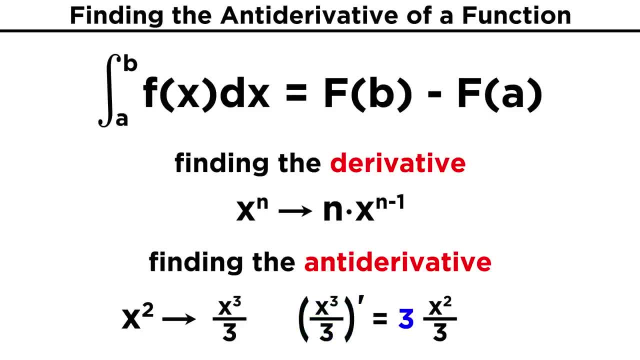 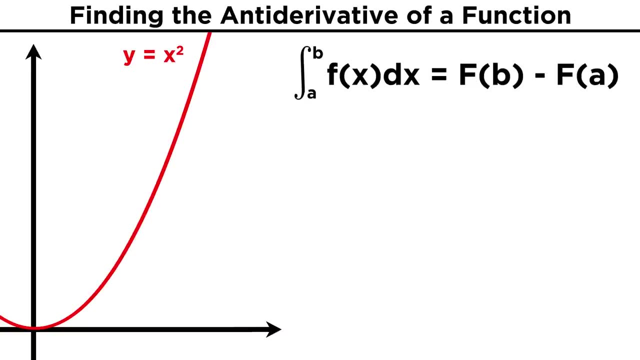 We can verify that this is correct by taking the derivative. Three comes down here and the exponent goes to two, The threes cancel and we are left with x squared, which is what we started with. So to contextualize this new definition of integration, 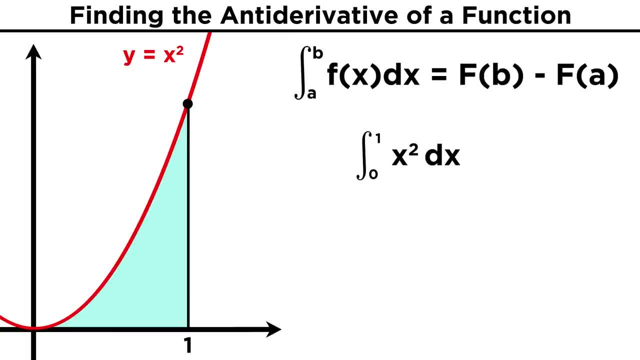 Say: we bring back the antiderivative, Let's take our x squared curve and integrate from zero to one That will be equal to the antiderivative evaluated at one minus the antiderivative evaluated at zero. That's what is meant by this notation, with either a vertical line or a closed bracket. 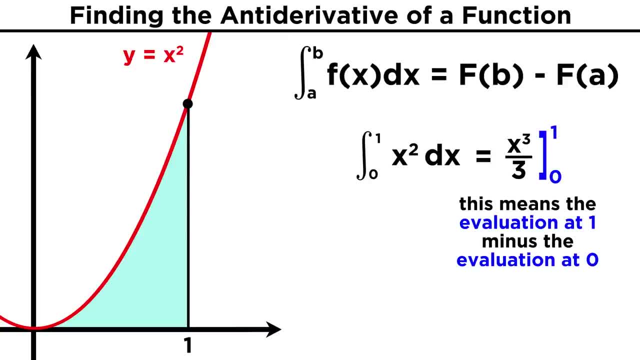 It means evaluate this function for the number on top and then subtract from that the evaluation for the number on the bottom. When x equals one, x cubed over three equals one third, And when x equals zero, it equals zero. So the answer is one third. 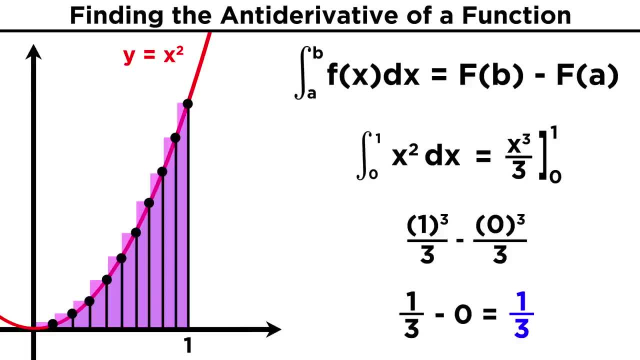 As we recall from the previous tutorial, this was the area under the curve that we got from the tiny rectangles, as the number of rectangles increased to infinity. So we can see that this approach of evaluating antiderivatives is doing exactly the same as. 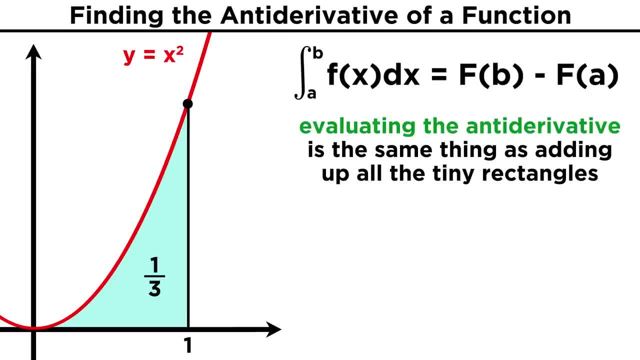 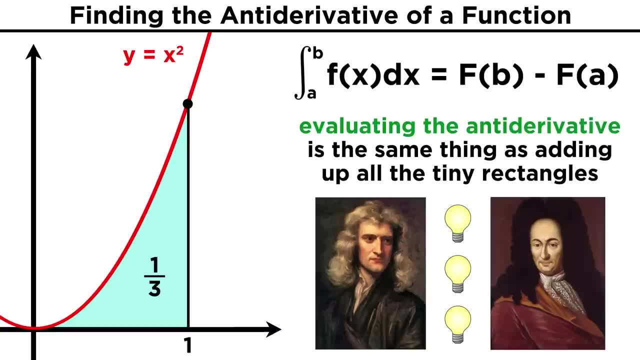 same thing, We are getting the area under the curve. This was the incredible light bulb moment experienced by Newton and Leibniz and their contemporaries in the seventeenth century. This was the realization that, just like addition and subtraction, or multiplication and division, 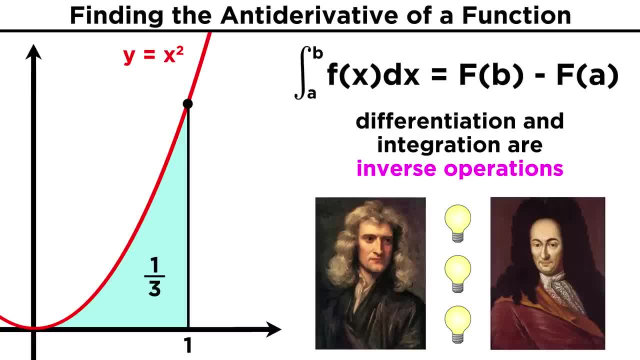 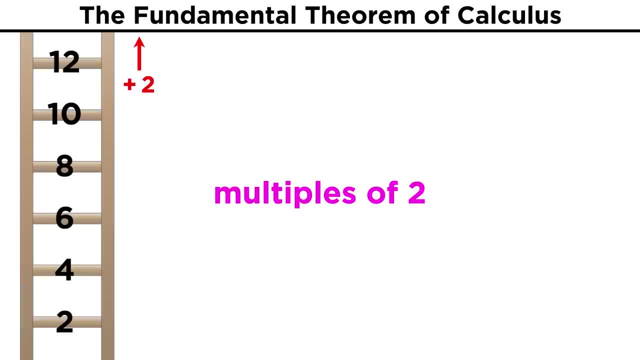 differentiation and integration are inverse operations. If we draw a ladder and on each rung we write a multiple of two- going up we add two every time and going down we subtract two every time. Addition and subtraction are therefore inverse operations. If we instead write the powers of two, then up represents multiplying by two and down. 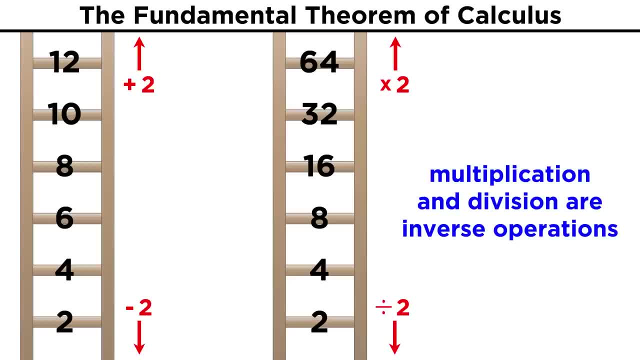 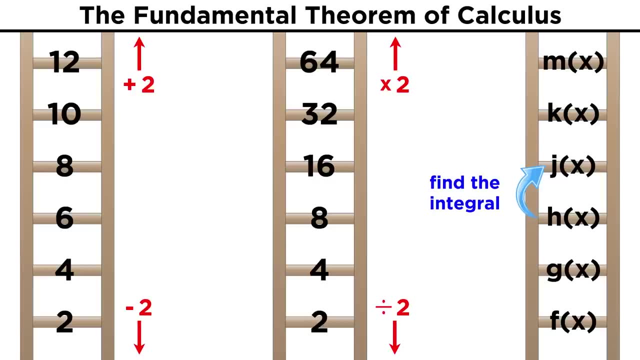 represents dividing by two. Multiplication and division are therefore inverse operations By precisely the same logic. if we write a series of functions on these rungs, each function is the derivative of the one above and the integral of the one below. The downward direction represents differentiation and the upward direction represents integration. 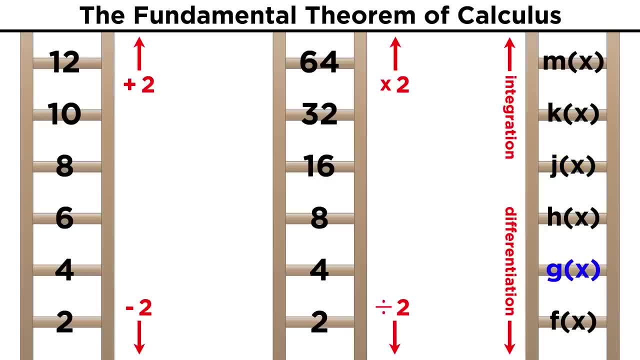 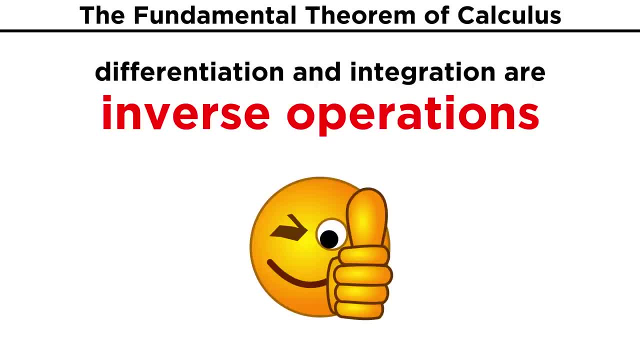 If we take the derivative of this, we get the one below. If we integrate this, we can get the one above. And this simple fact- the inverse relationship of these two operations- is the integral of the one above. This is the essential truth that we refer to as the fundamental theorem of calculus. 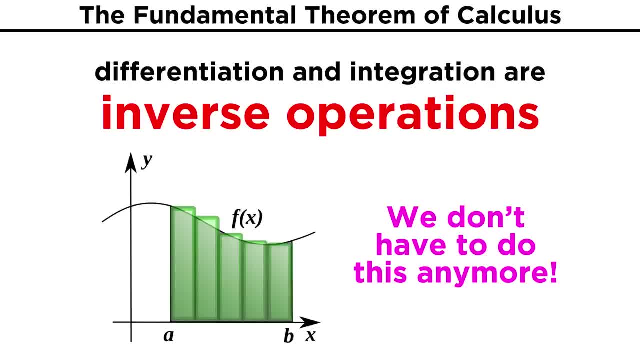 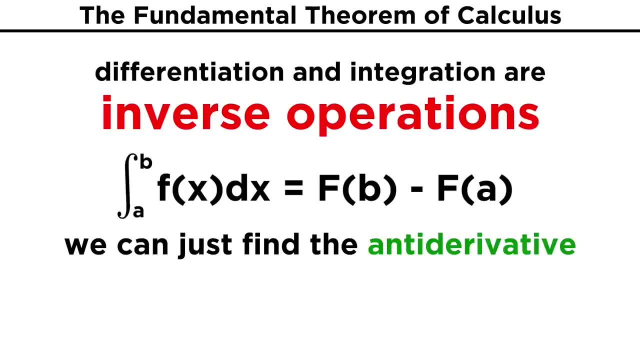 This new understanding means that integration can now be thought of not as the obsolete approach of constructing tiny rectangles and finding the limit of a sum, but rather as an entirely new computational algorithm that is simply the inverse of differentiation. The derivative of the integral of a function is just that function, in the same way that 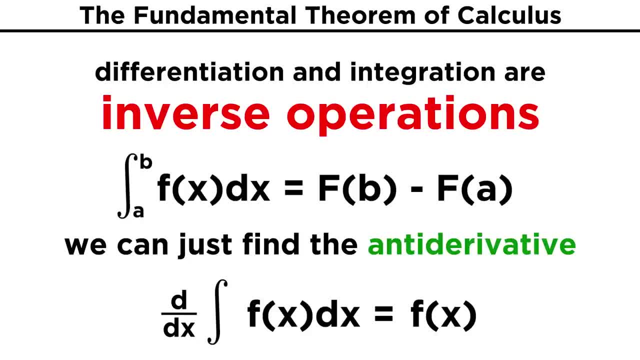 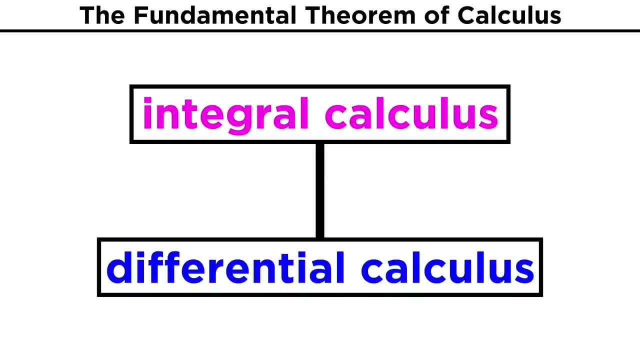 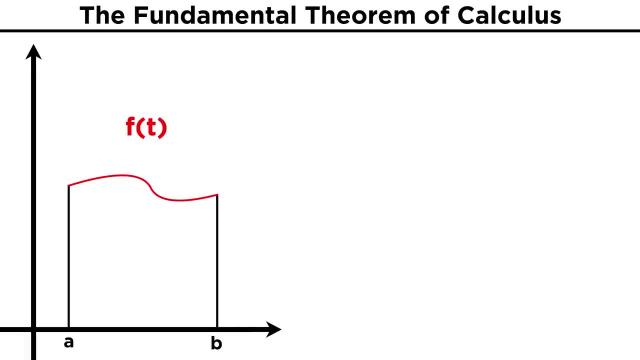 the square of a square root gives us what's inside the root. Integral calculus and differential calculus are united at last. Now that we have a basic grasp of this theorem, let's express it a little more formally. We have some function f of t which is continuous over the interval from A to B. 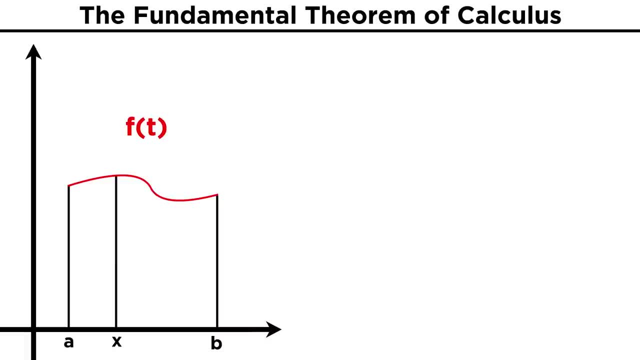 If we want to integrate this function from A to some interval x, we get a new function, g of x Equal to the integral of f of t, dt from A to x. Notice that this new function does not depend on t, but only on x, the upper limit of integration. 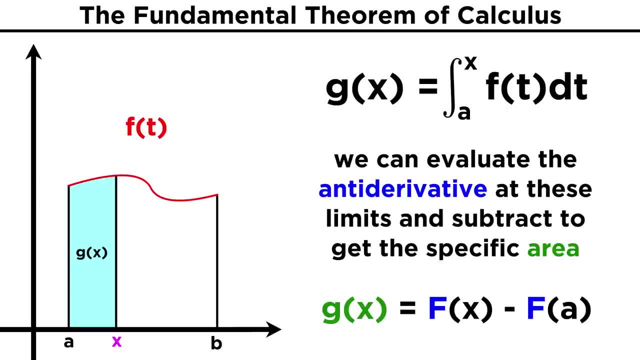 If x is a specific number, instead of getting a new function, we would use the antiderivative of f and evaluate for the limits of integration to get a number. This would be the area of this section under the curve. If we leave x as a variable, then we instead just get the function g of x. 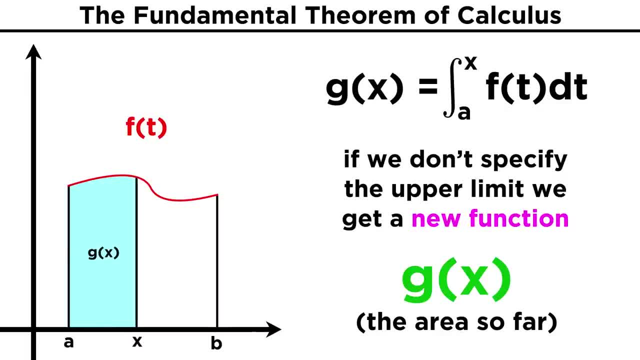 We can think of g of x as the area under some section of the curve, depending on x, or the area so far as x moves along the curve, As we just learned, it will be the case that g prime of x will equal f of x, and that means 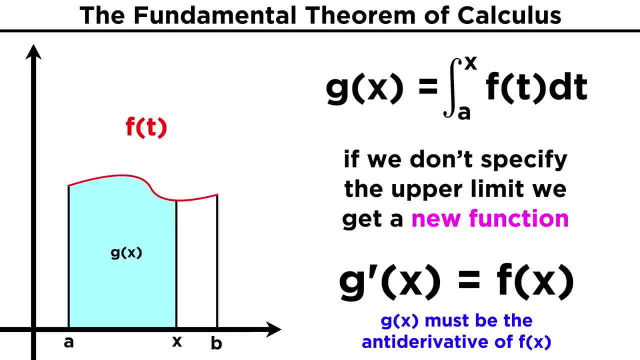 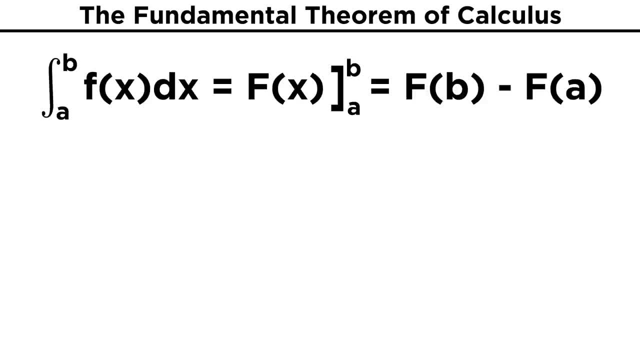 that g of x must be the antiderivative of f of x. This brings us to the second part of the fundamental theorem, which is the algorithm we mentioned earlier. The integral of some function, f of x, dx from A to B, equals the antiderivative of f uppercase. 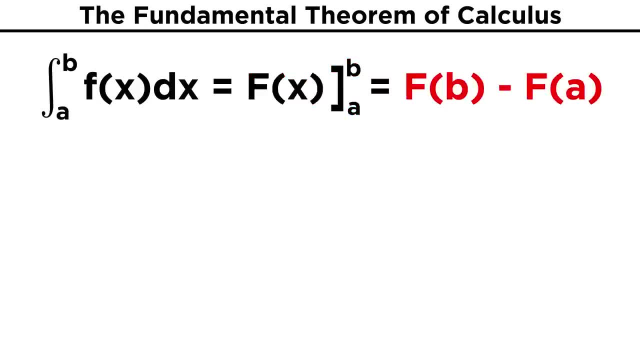 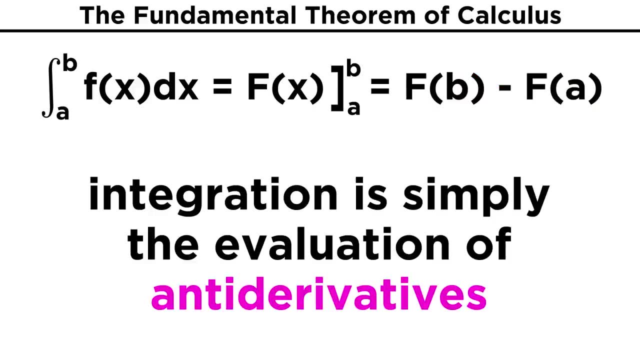 F evaluated over this interval, which can also be expressed as the antiderivative of B minus the antiderivative of A. This is our new way of thinking, Thank you. This is our new way of approaching the evaluation of integrals, so we won't be talking about. 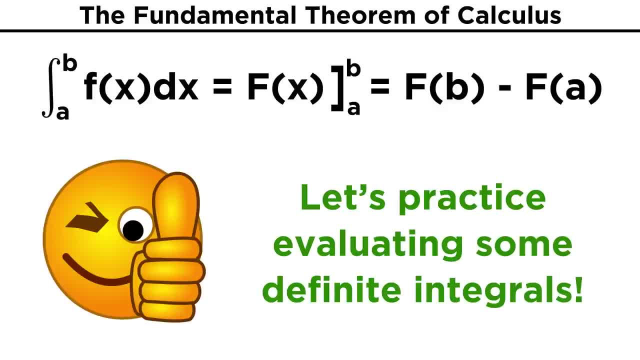 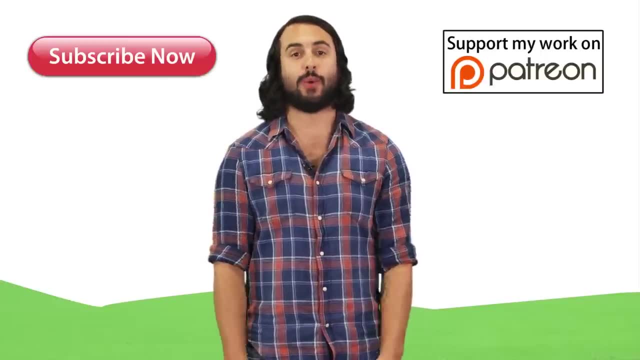 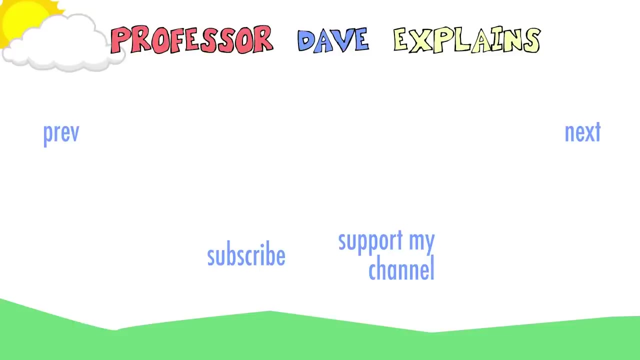 rectangles anymore. Now that we have this theorem under our belts, we are ready to practice evaluating definite integrals, so let's move on to that concept next. Thank you very much for your attention and I hope you enjoyed this video. We will see you next time. Bye.